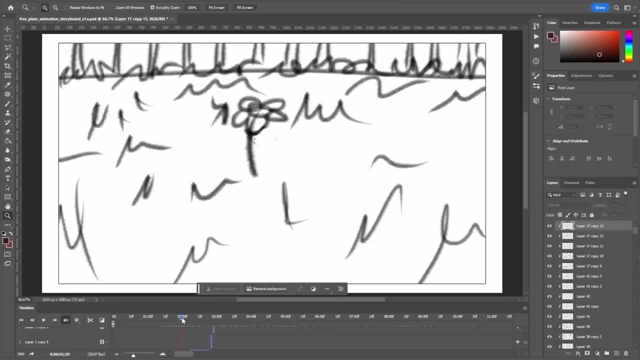 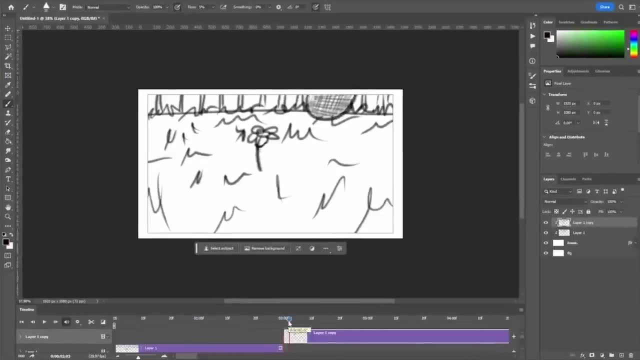 actually make sense in the end. But Pixar doesn't stop there. They also animate the individual shots very roughly, which means that at the end, you basically already have the whole movie planned out. This step is tedious. it takes a long time, but now I know that the animation is around 3. 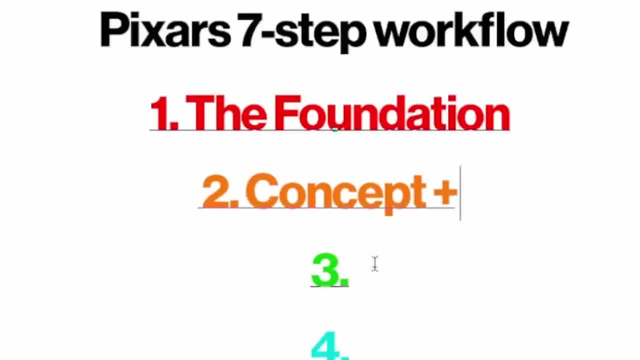 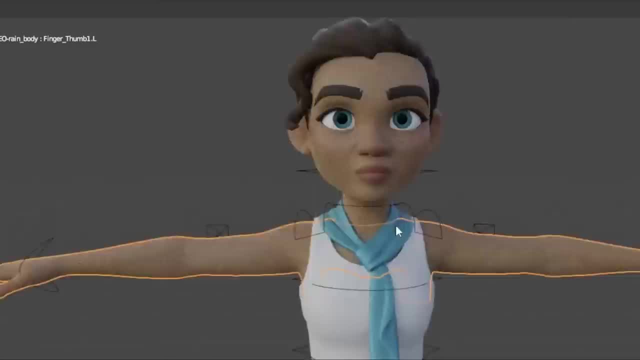 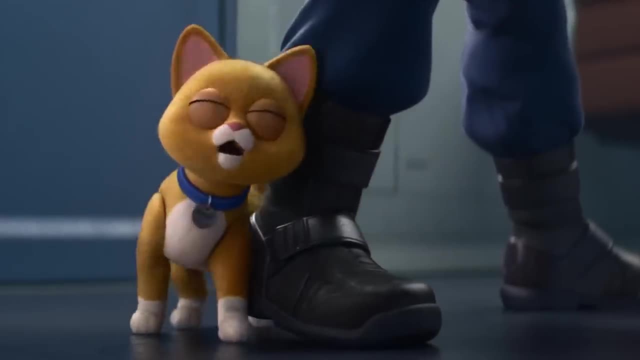 minutes long and I better start working on it In step 2.. The concept and design phase: To create a unique look and feel with unique characters and environments for every animation. Pixar has a team of concept artists that design all the characters and environments. I also have a team. It's called the Blender Studio. 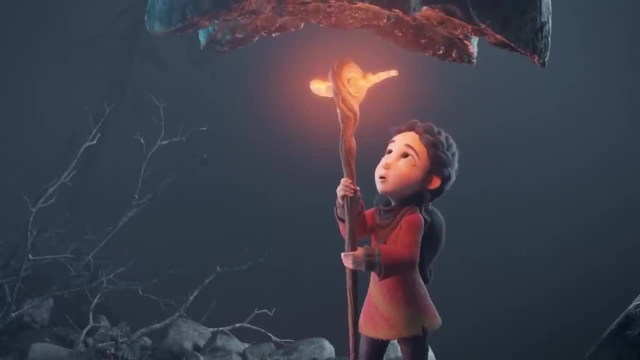 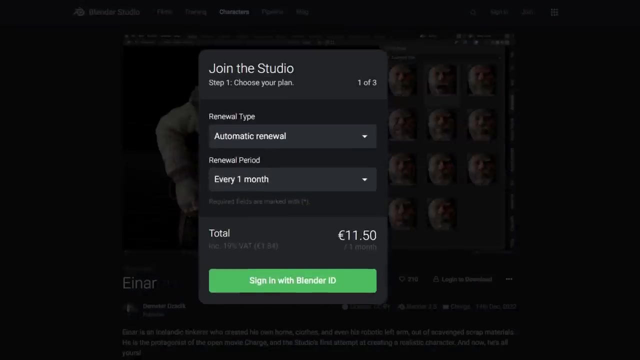 Character Library. The Blender Studio has created a bunch of animated films over the years, and most of the characters from those are accessible in this library. For some of them you have to buy a membership, but for some, which stylistically work pretty well together, you don't Plus. 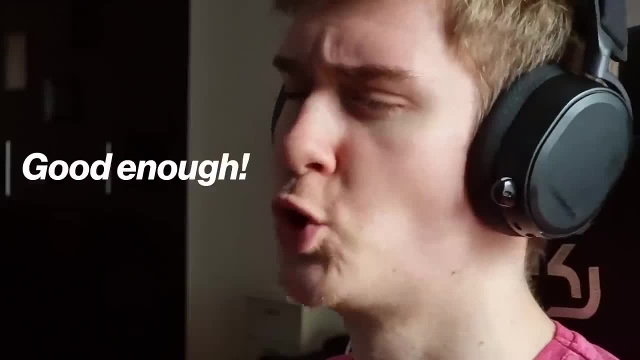 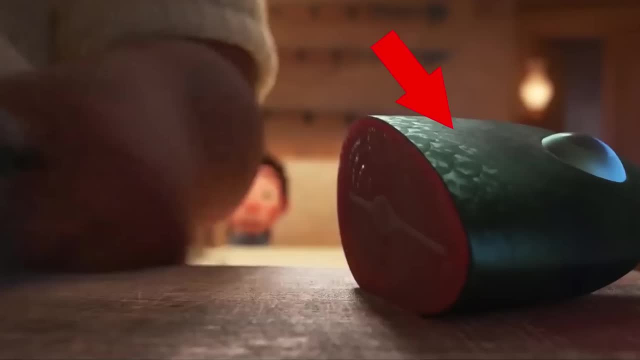 they also look pretty similar to the Pixar style, so that worked out pretty well. Say hello to snow, rain and autumn In general. the Pixar style is basically a combination of stylization and realism. All the objects in the world are stylized, but the details of those objects are realistic, So 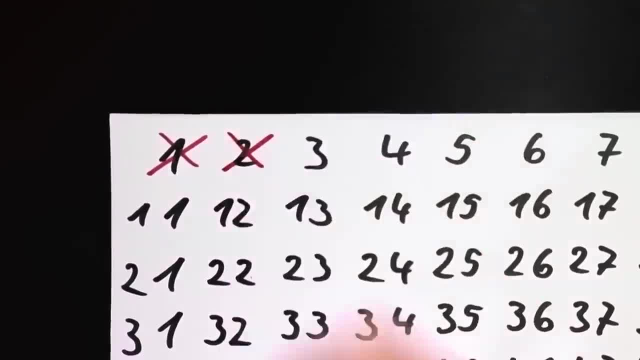 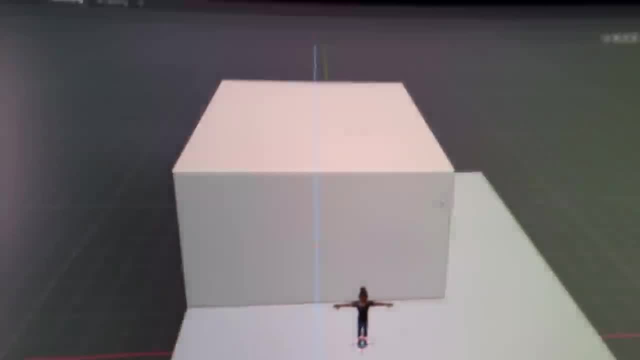 with the characters ready to go and Pixar style in mind. it was day 3 and I was ready to start with step 3.. Building the world With my storyboard in mind, I blocked out the environment. The first goal was to make it functional, And with functional I mean work for the animations I had in mind. 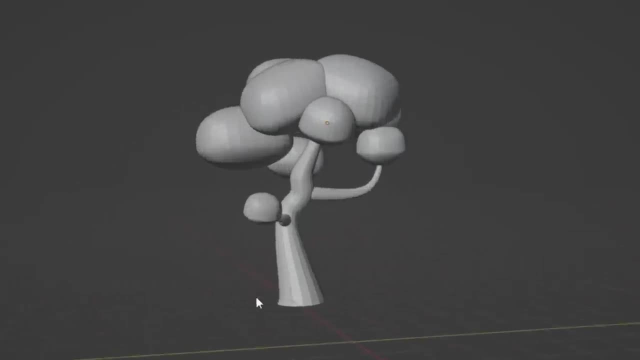 Some scenes need a house, Some other scenes need a tree, And to make the surrounding environment more appealing, let's start with the tree. So I'm going to start with the tree, And then I'm going to add a whole neighborhood, And now, with the block art of the environment in place, I went to 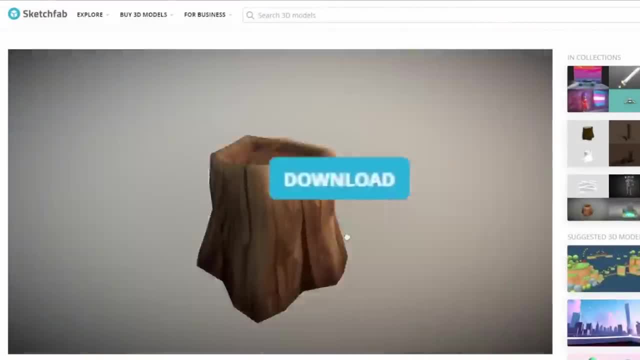 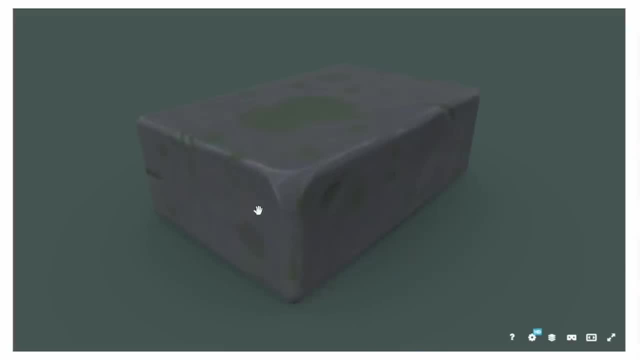 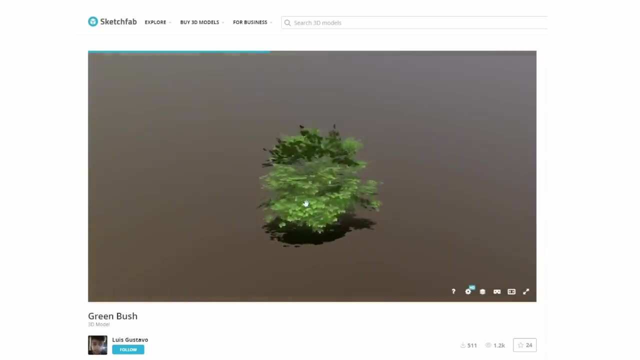 Sketchfarm to see if I could find some fitting free models that I could use to speed up the detailing process. This model, for example, had a nice fence for the garden and flower pots for the windows. Or this bush, which I used all over the garden, including the tree. 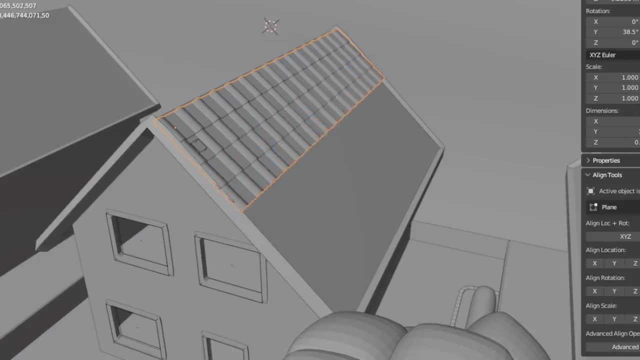 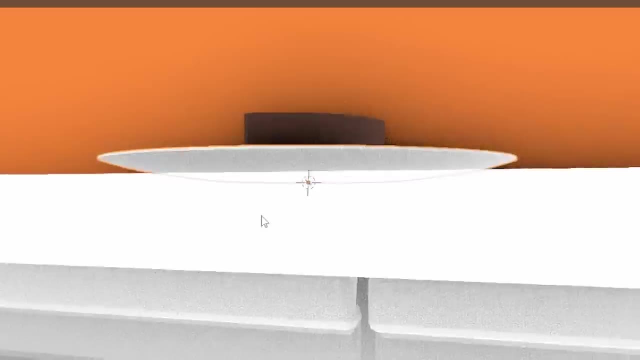 The goal was to refine the fundamental elements first, before I later refined the rest, Which is also why in this first part of the project the pie, for example, still looks like a brick. So don't complain later, when you see the first part of the animation, that the pie is still unfinished. 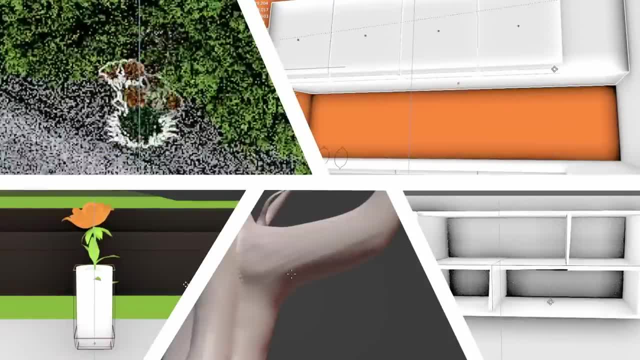 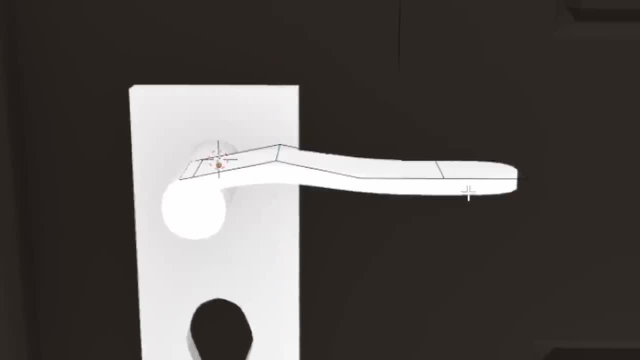 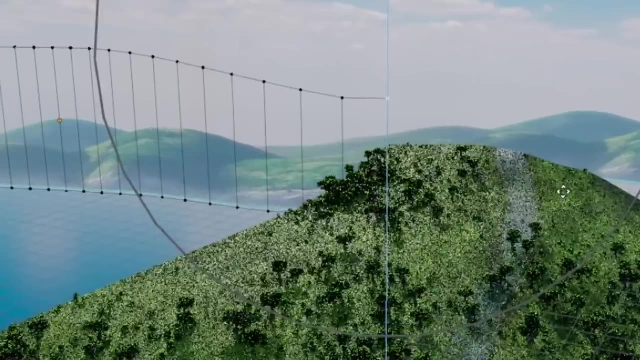 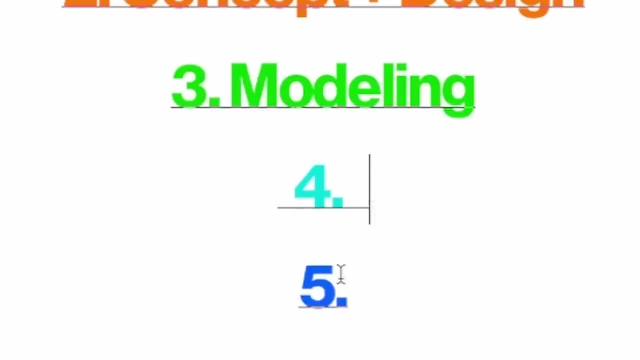 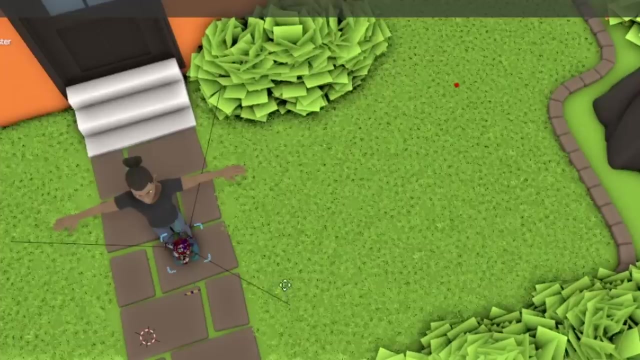 okay, Haha, Okay. with all the essential elements in place, day five is rolling around and it is time to animate. Well, sort of. It's pretty clear by now that before every complex step, there's a step that makes sure that nothing goes wrong. We don't want our actors to hurt themselves, so why would 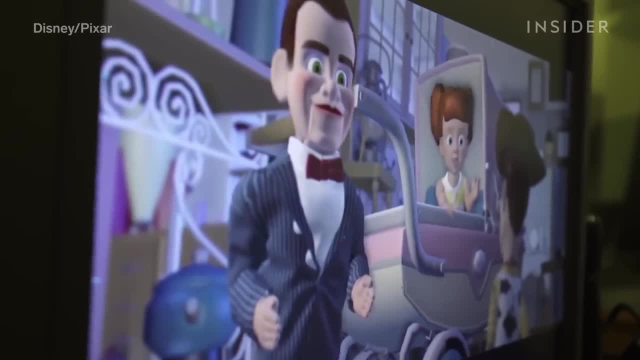 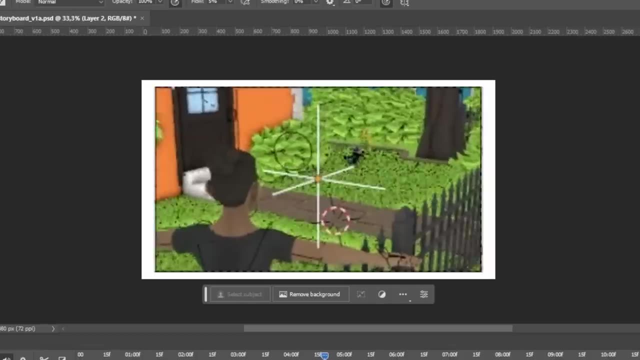 we break that rhythm now. Before they really start animating, Pixar likes to block out all the shots first. For me, that basically meant trying to decipher the scribbles I drew a few days ago in my storyboard and recreating them in 3D. 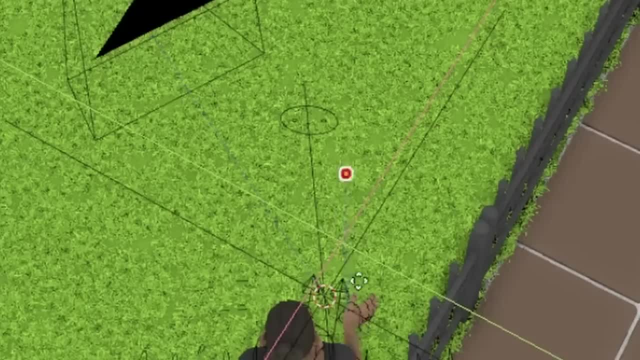 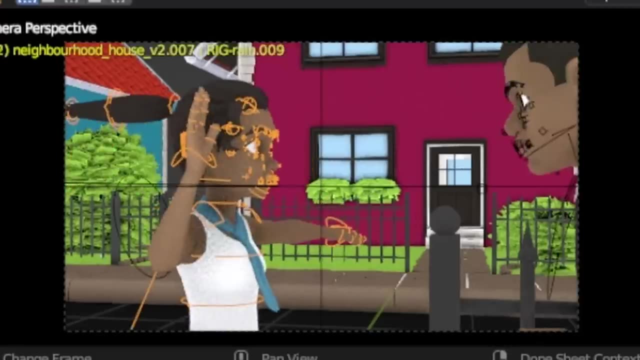 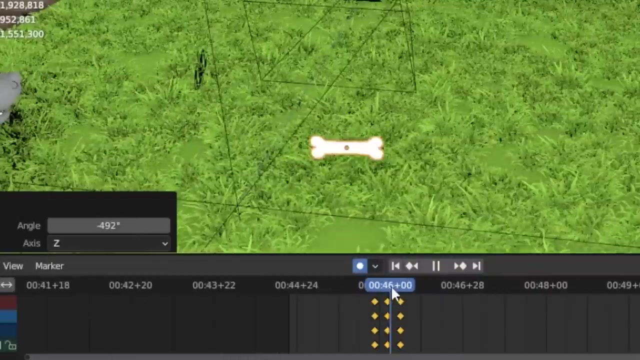 This seemed like an unnecessary step at first, but it allowed me to focus on the cinematography and timing first, before I need to care about the exact movements of each character. The scenes are set, so now it was finally time to animate. Animating basically just means changing. 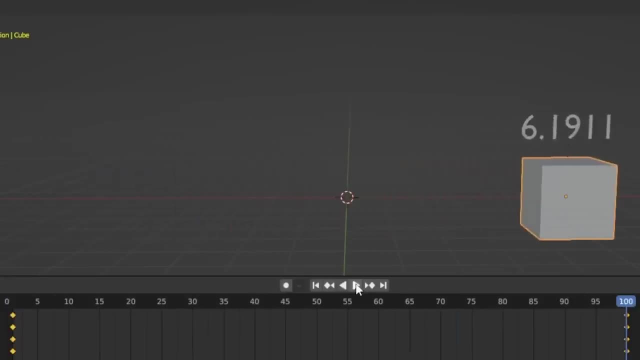 a value like the position of an object from one point in time to another. So if I wanted to animate snow raising the height of snow, I would have to do that first. So I'm going to do that first. So if I wanted to animate snow raising his leg, I would mark this pose, move forward in. 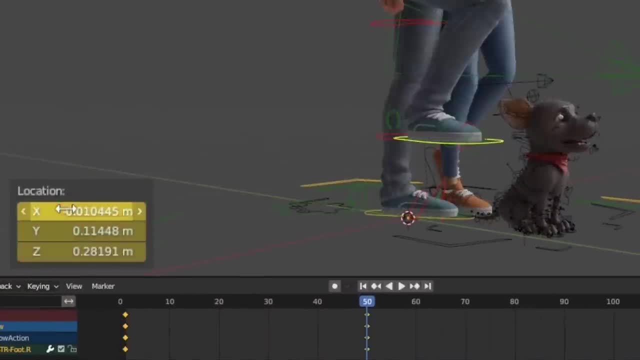 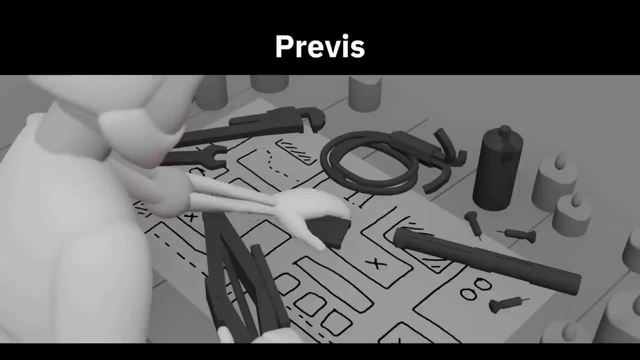 the timeline, raise his leg and then mark this second pose, And that's how basically everything gets animated. From what I've seen, most character animators create all the most significant poses of a scene first, and afterwards they refine it to make it look more natural, And that's how I did it. 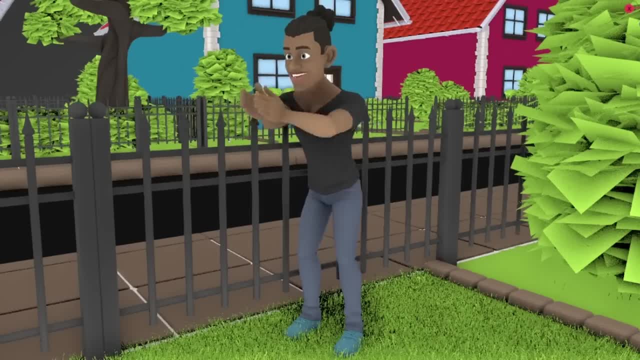 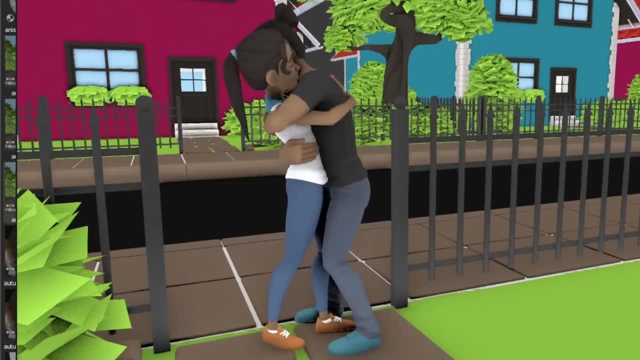 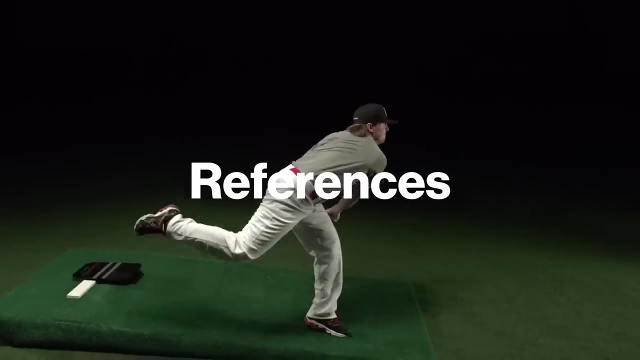 too. Basic poses: refining final animation. Basic poses: refining final animation. Basic poses: refining final animation. Out of this process, I also learned to love two things in particular. The first one is references. If you're trying to create realistic animations, you might as well use realistic references To. 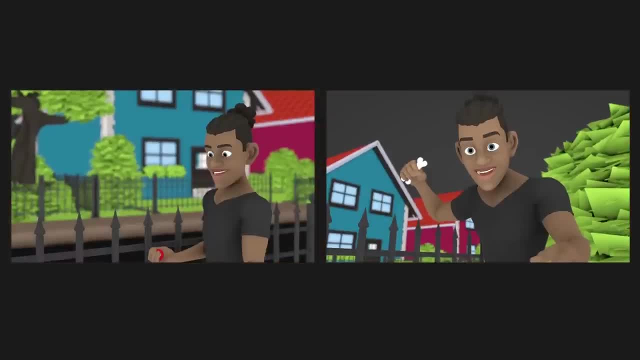 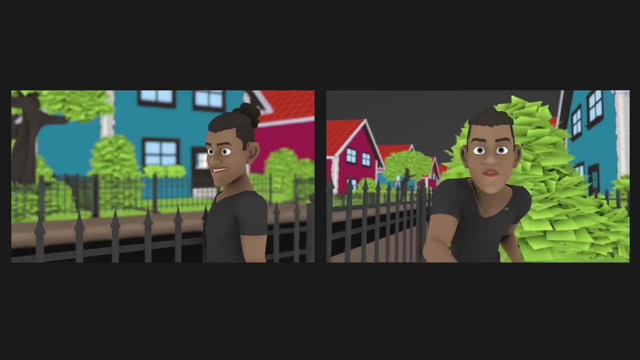 show you how much of a difference this can make. look at these throwing animations. The first one I made without reference, the second one I made with reference. I think the difference is pretty obvious. And if you can't find fitting references on the internet, you can also just shoot it. 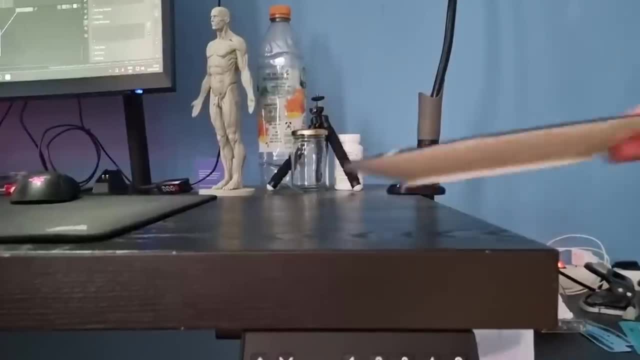 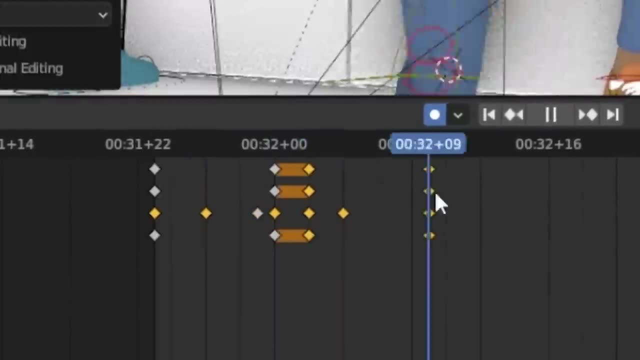 yourself For this scene. for example, I shot myself putting a plate on a table to see how I move my fingers. The second one is the graph editor. Basic keyframes can only get you so far. The graph editor allows you to adjust the flow at which the values of your model are being changed. 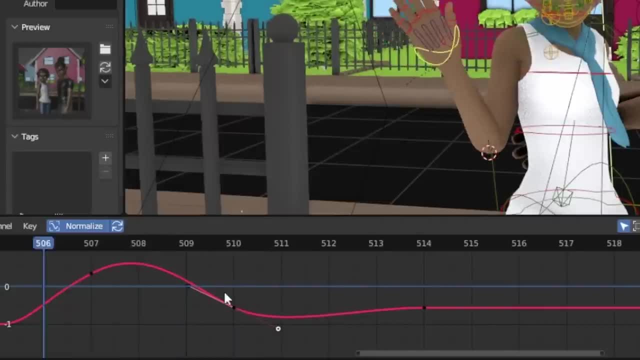 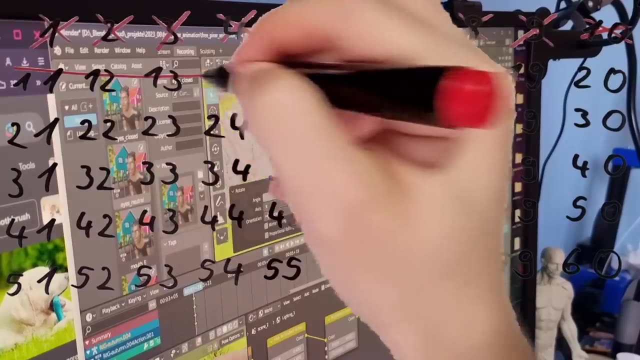 This can be super helpful to create more bounciness in your characters or to just smooth out their movement. Before the graph editor. after the graph editor: It is quite a tedious process, but it's also just as satisfying to see the characters move. 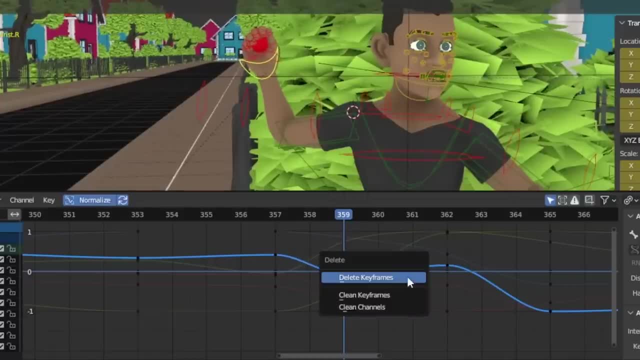 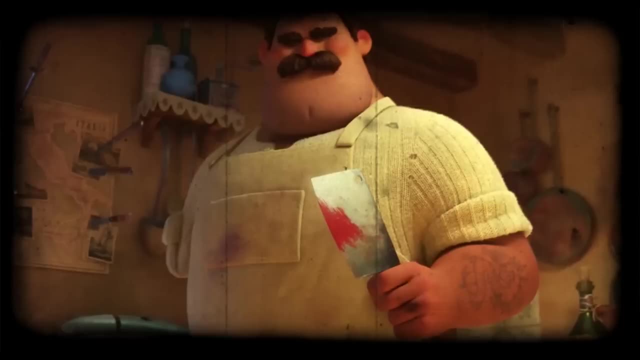 just how you've imagined. once you're done- Or at least almost as you've imagined- I might go back and fix some of these later if I have the time for it. But with the animation done, there were only two more steps left. Earlier I described Pixar's style as basically a combination of stylization. 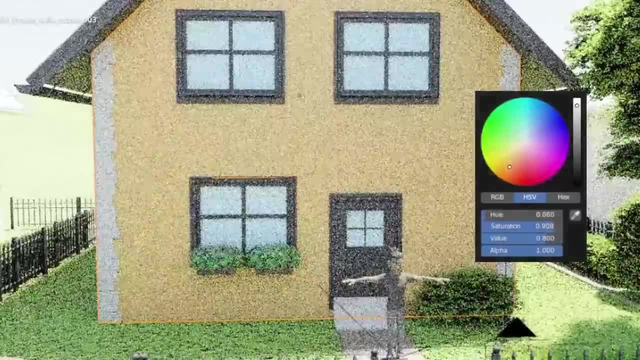 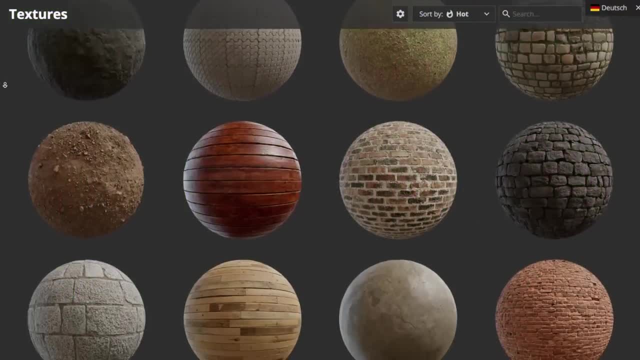 and realism. So far, I only really color-coded most objects, so now it's time to add some nice details. The bark of the tree, the wooden floor, even grass, got a new look. For most of the objects, I used three realistic textures, while for others, like the tree, I credit my own with Blender's. 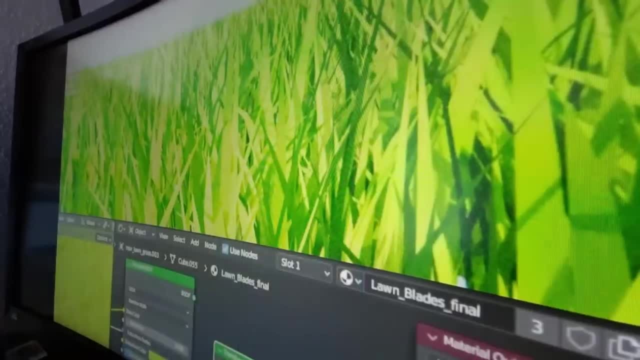 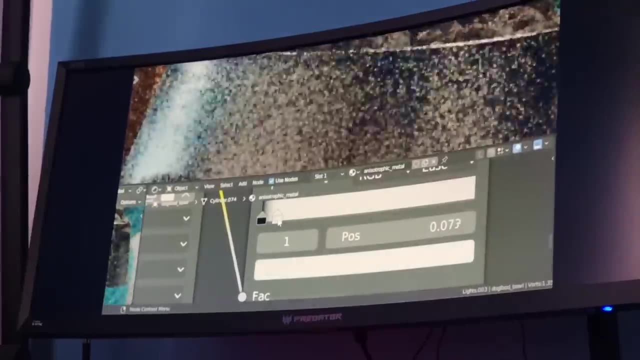 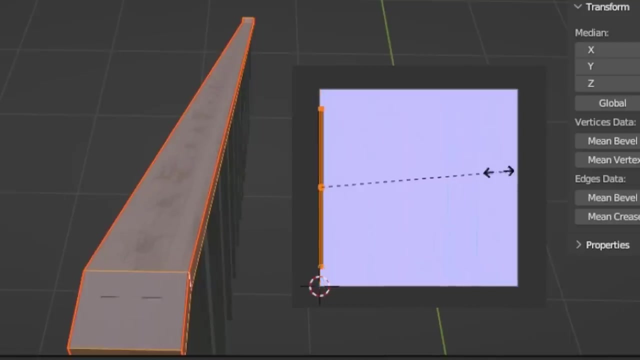 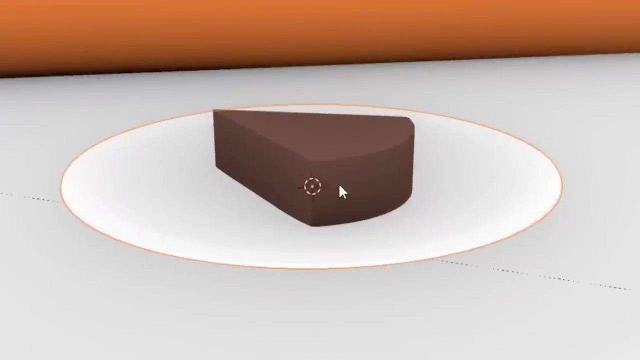 internal textures. I've only refined some objects so far because I wanted to focus more on the last step, but in the end almost everything will have a nice detailed surface like this. So once again, the pie will look better in the end, I promise. 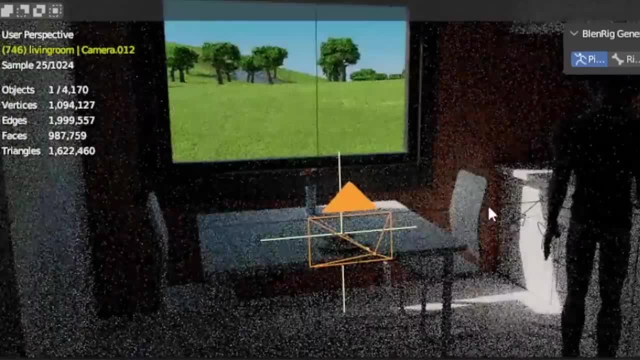 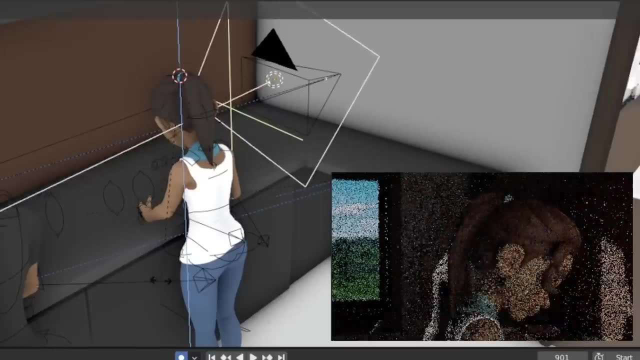 Now, this last step actually blew me away Here. let me actually just show you what it is Before After. It is just so good. For the second one, I added a few more extra lines which realistically wouldn't be there. 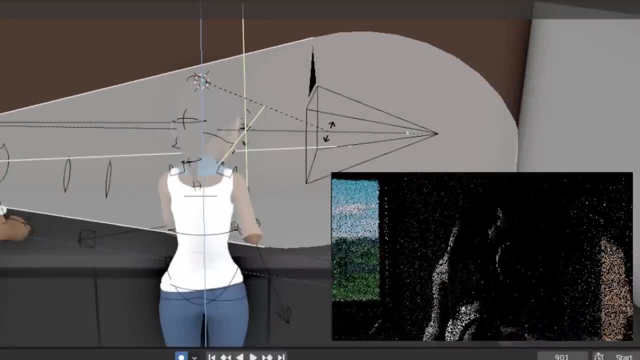 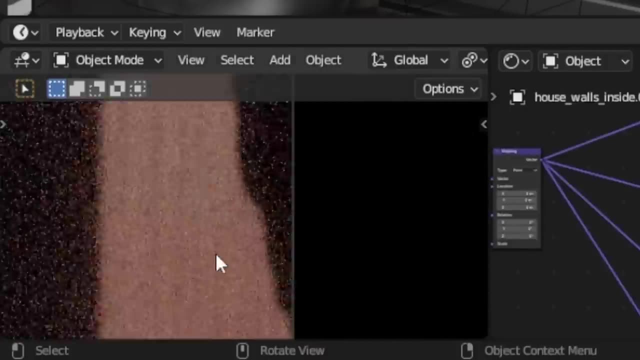 but they add so much more flair and clarity to the scene that it's more than worth it. And as long as the lines are strategically placed so that they make sense, it can only really help the shot. The sun here, for example, is shining through the window onto this wall, so I placed 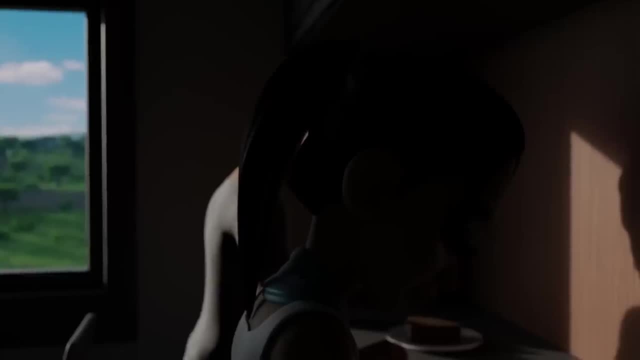 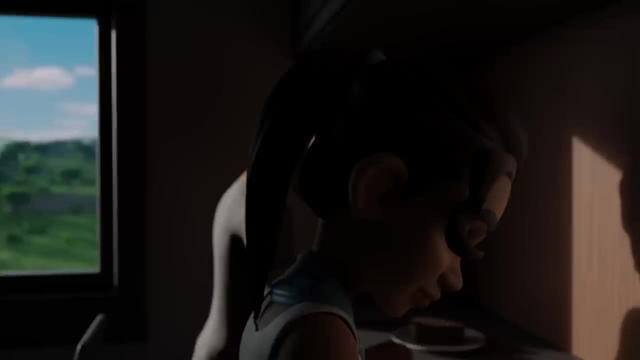 a light shining onto her face from that direction which just slightly illuminates her face. The light from the sun doesn't actually hit her at all, but you can see that through the camera, so it looks like it makes sense. adds so much more contrast to the scene. 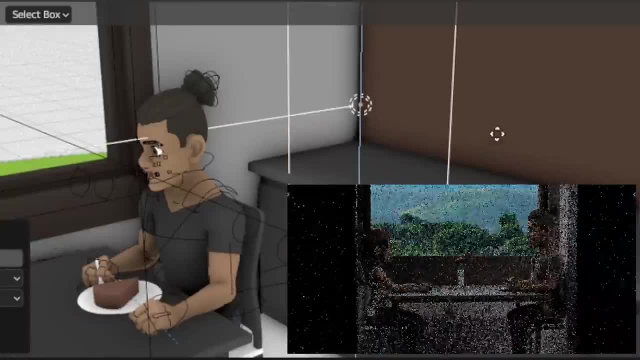 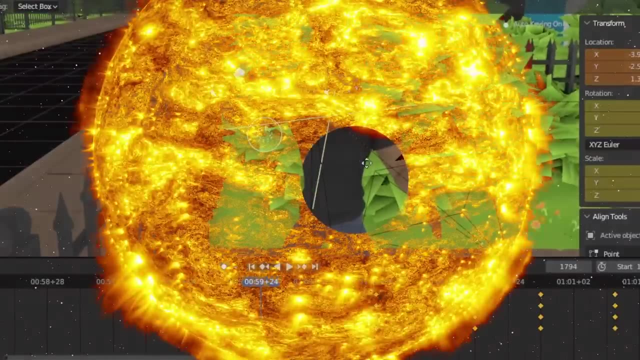 and perfectly sets her apart from the background And after lighting and all the necessary shots in that way. 25 days have already passed. This project felt really scary. before I started, I was working on a different project before this, where I encountered a problem that I just couldn't find a solution for. 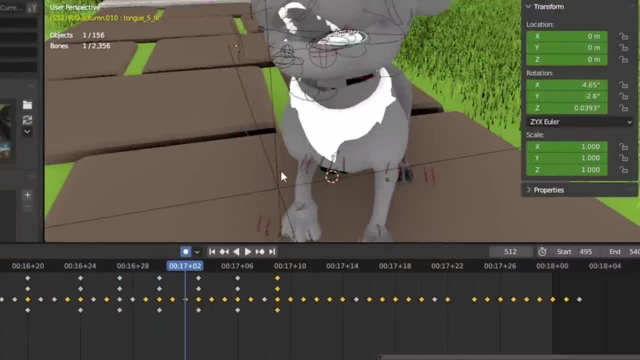 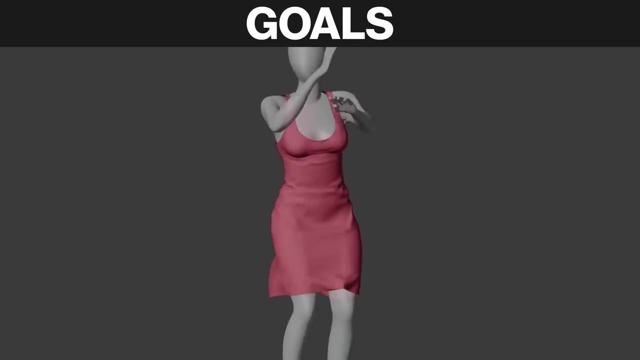 so I had to give up on it And I was kind of scared that that was gonna happen for this one as well. But following this step-in-step workflow made it actually pretty approachable. The goal for the second half of the animation are to add a cloth simulation, adding more scenes with 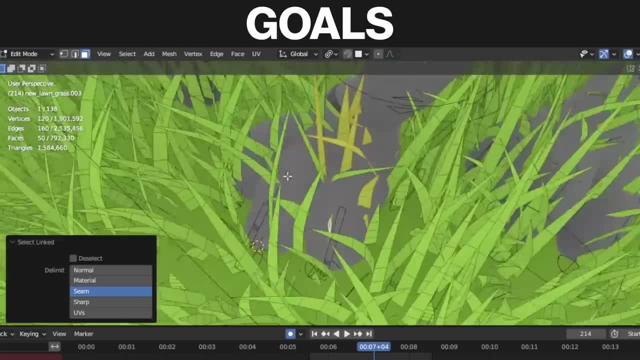 different moods and lightings to create different emotions, hopefully making the grass reactive to people stepping on it, and then adding more scenes with different moods and lightings to create a different atmosphere. And there's gonna be a fourth character joining the squad. 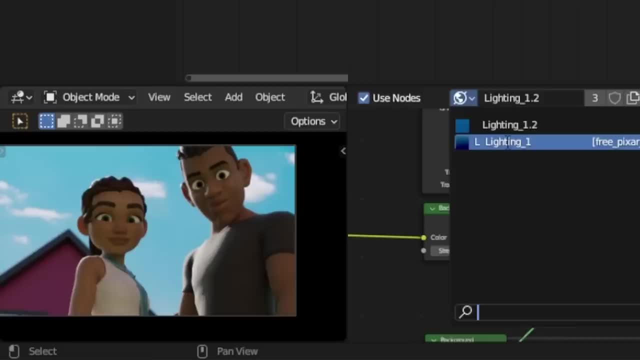 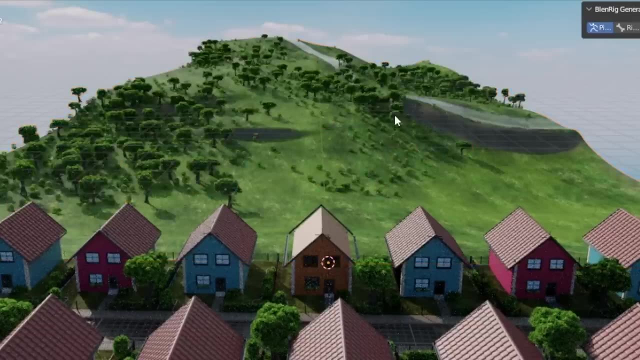 So some new and scary stuff coming up, but so far I would say, yes, you can create an animation like Pixar on your own, But we'll see how the rest turns out. To end this video, here's the first part of the animation, not finished, but pretty far down the 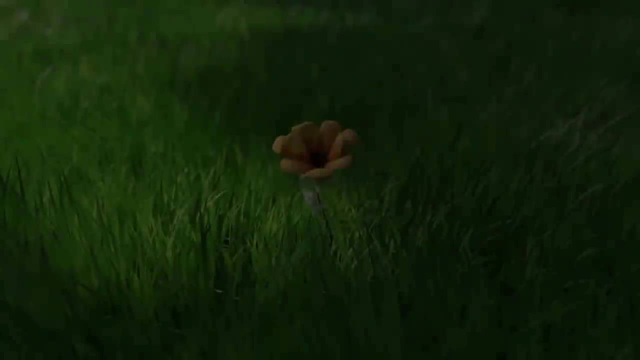 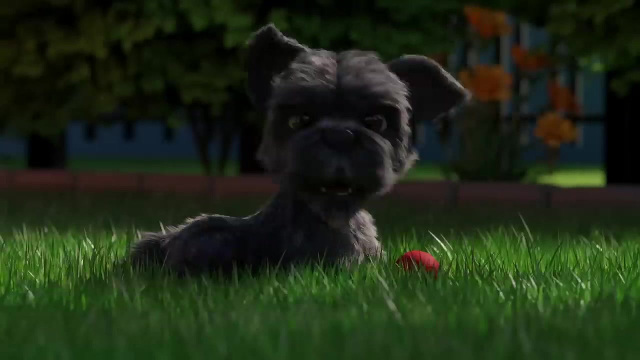 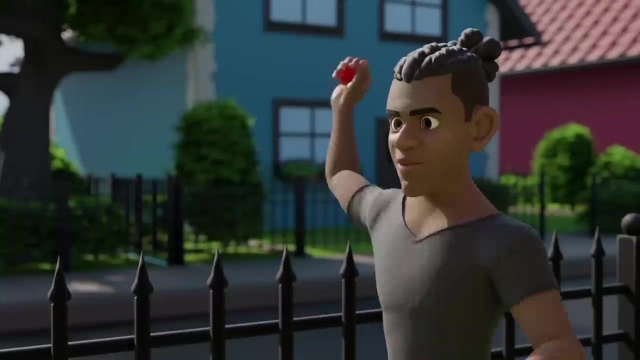 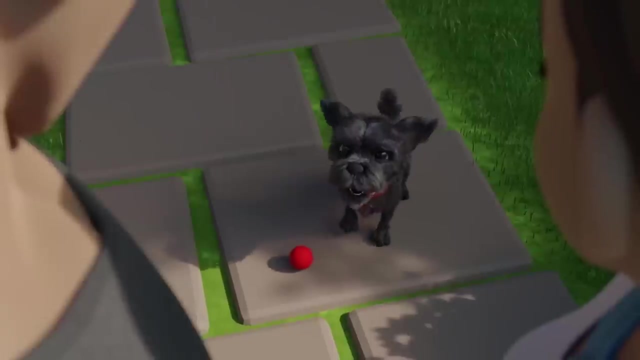 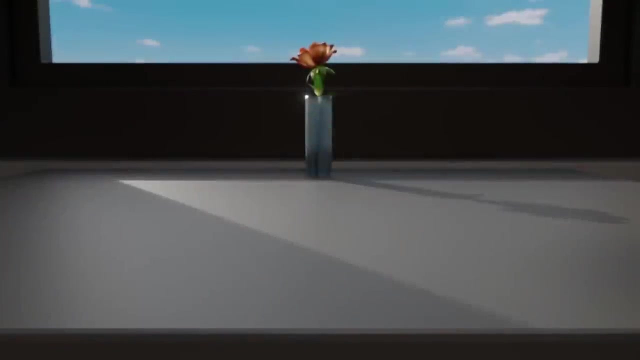 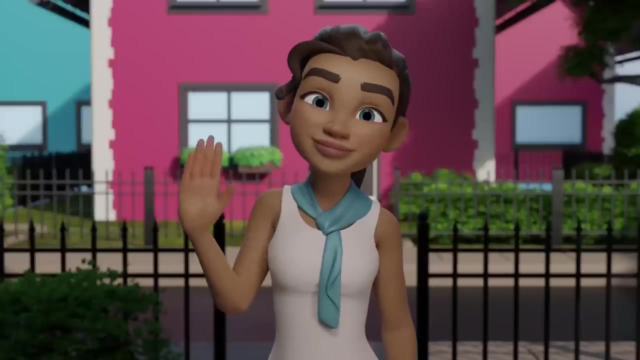 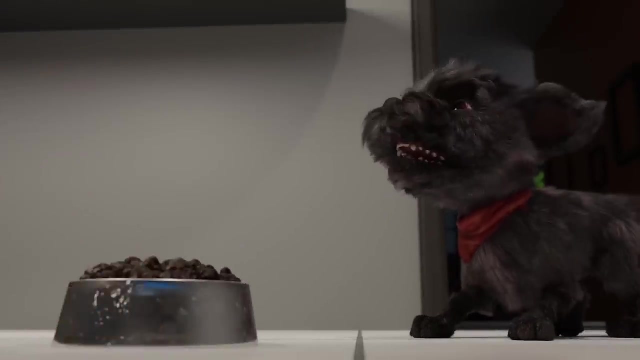 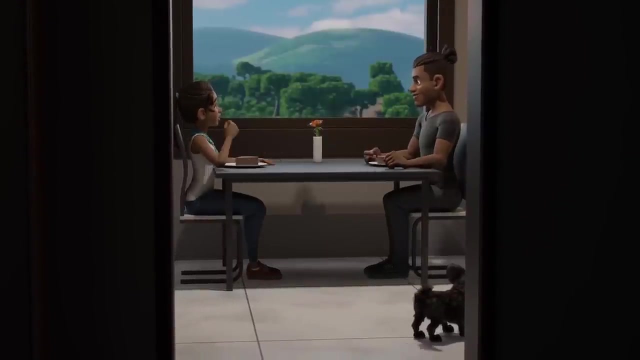 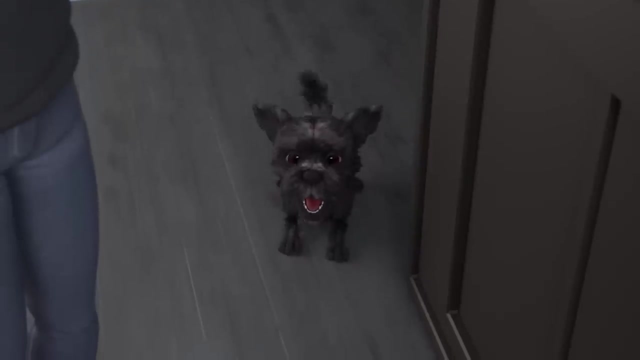 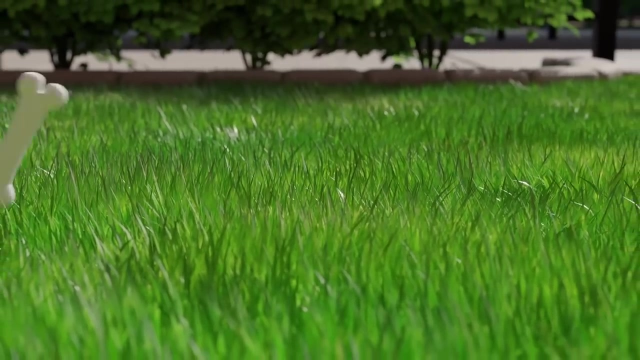 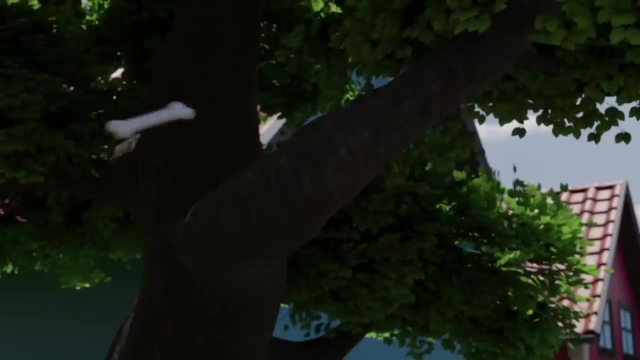 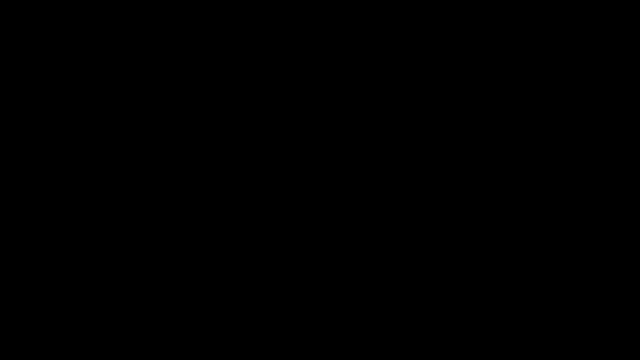 line: you want your ok home and what and? and Thank you, Thank you.